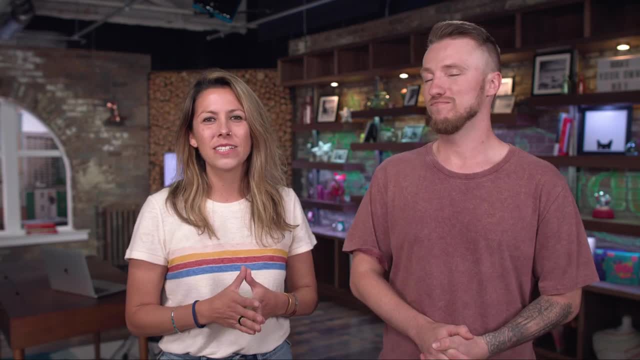 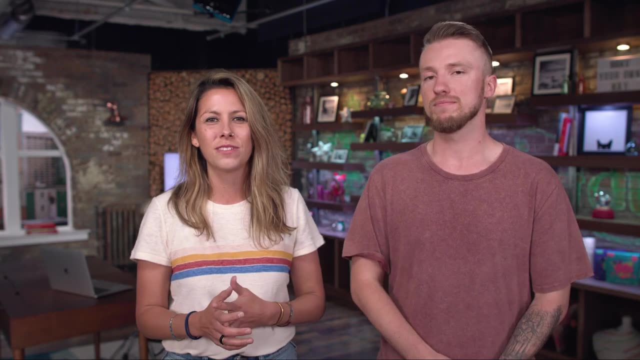 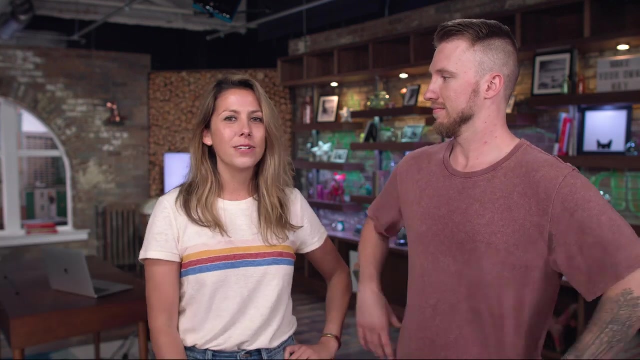 lesson. It's a tough lesson. So, first off, listen. And your customers. they're out there, messaging you on Facebook, Mentioning you on Twitter, leaving reviews on Yelp. So customer service tip number one: listen to them, Don't ignore them. You wouldn't do that if I walked into your shop today and I was like: 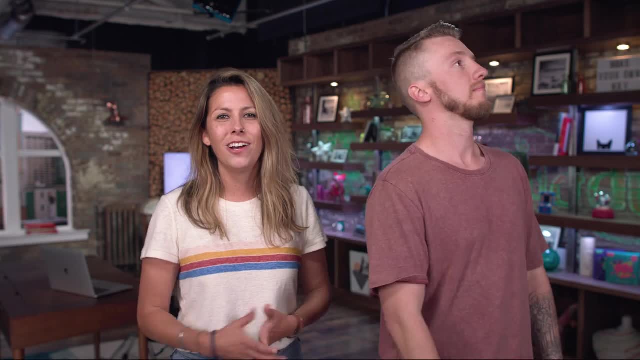 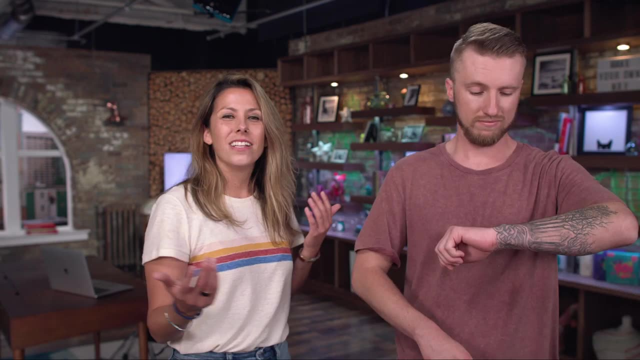 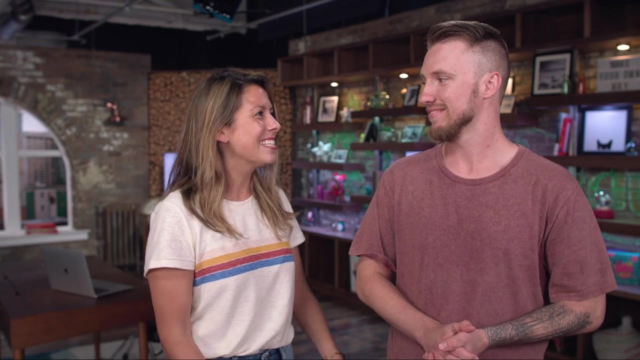 hey, Justin, you make a really great cup of joe. I love coming here, Justin. I love coming here all the time. Thank you so much. You know what I mean. Like you don't ignore that person, You don't, You would acknowledge it like this: Hey, what's up, I love. 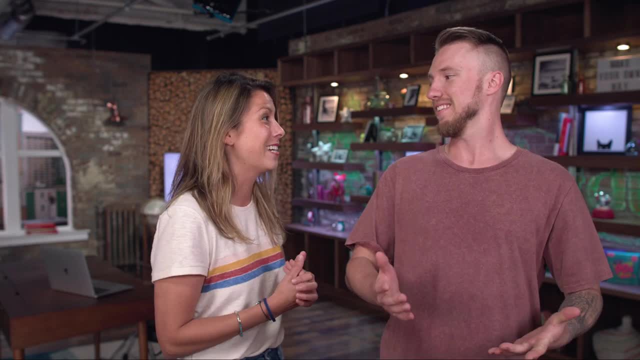 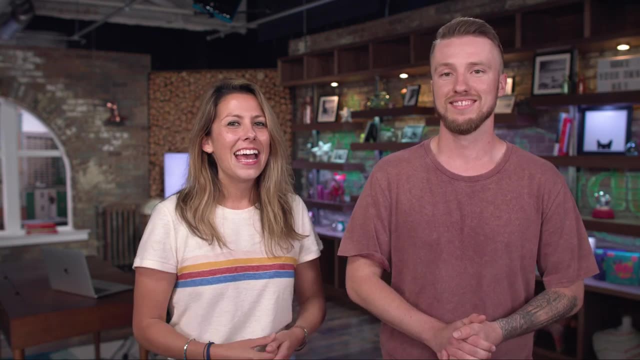 coming here. Your cup of joe is the best in town. I've been coming here for three years. I love it. That is so awesome to hear. I appreciate you coming in Bingo, So listen. And then that leads us into tip number two: always respond. 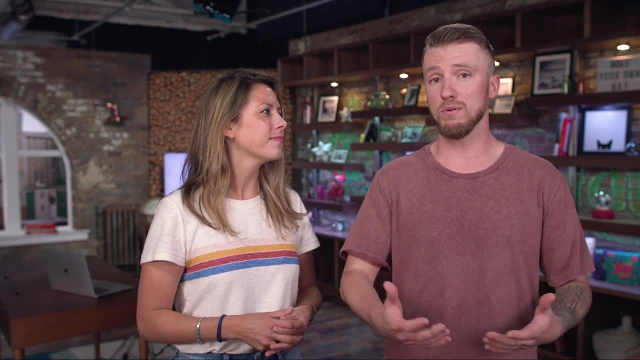 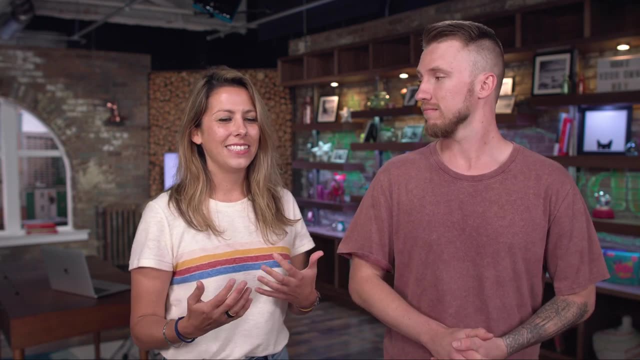 Yes, Always respond. Even the negative comments, always respond. What are your tips with responding? So be very personalized in your response and definitely do it in a timely manner, which is tip number three, because you don't want to let it just. 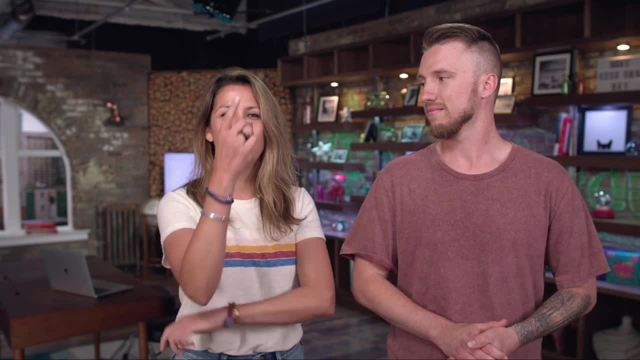 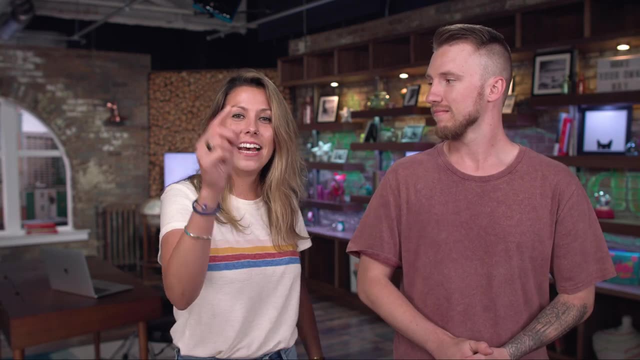 hang out on your page, because then more and more people are going to see it and wonder: Do they exist? Are they alive, Are they still in business? Where are they Exactly Like? why isn't this person responding? That's your customer service online. So again, 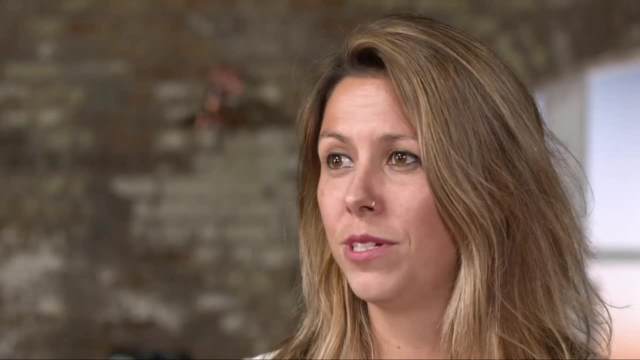 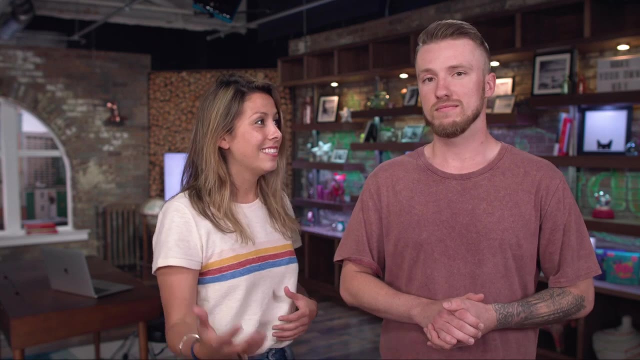 do it the same as you would in your business, Okay, So, when it comes to responding, I know I said do it in a timely manner. What is timely? Yeah, What's timely? There was a study, because we nerd out on this stuff all the time. There was this study that said two out of 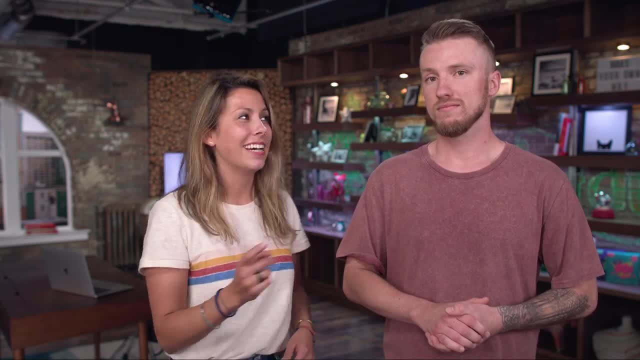 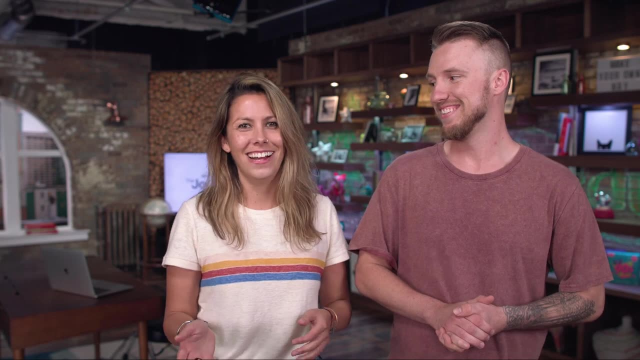 three consumers respect a response. Guess, just guess, Guess, Yeah Within I cheated. I know the answer. He does this a lot 24 hours, 24 hours, And if you're on Twitter and you get a response there, 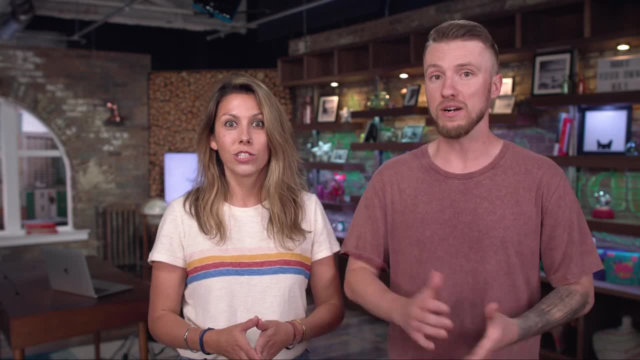 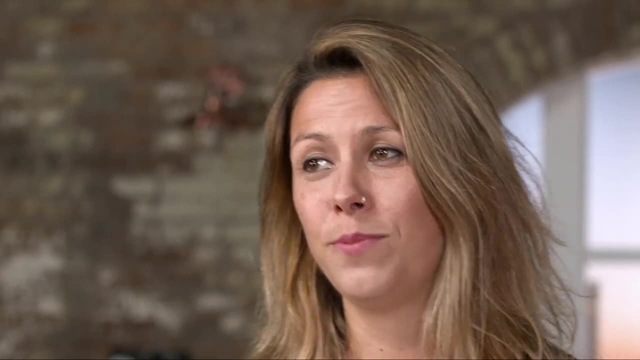 they actually expect it within two hours. It's crazy, right Crazy. So the point is be timely. So we've talked about listening, We've talked about responding and then, of course, responding in a timely manner. That leads me to number four. 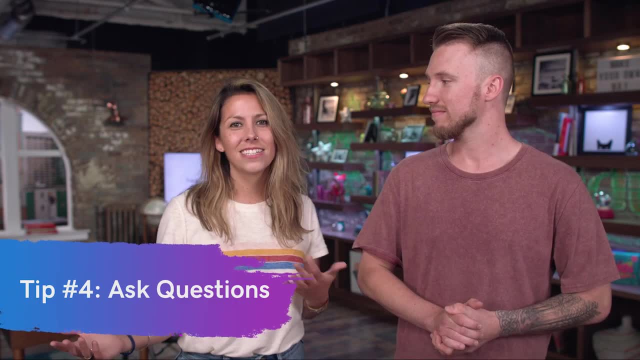 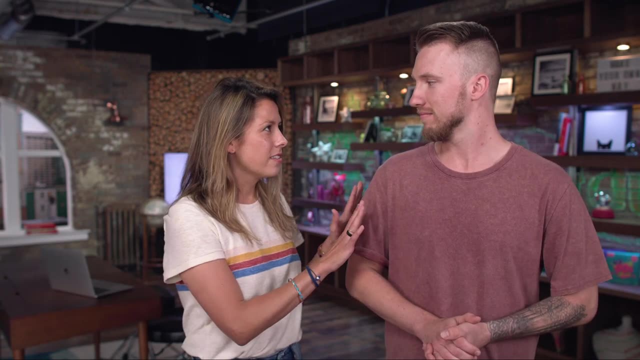 Number four: ask questions. This is a great chance to get to know what's working, what's not working, what your customers love about you, Maybe what they want you to work on Right. Take the criticism. It can help you in the long run. 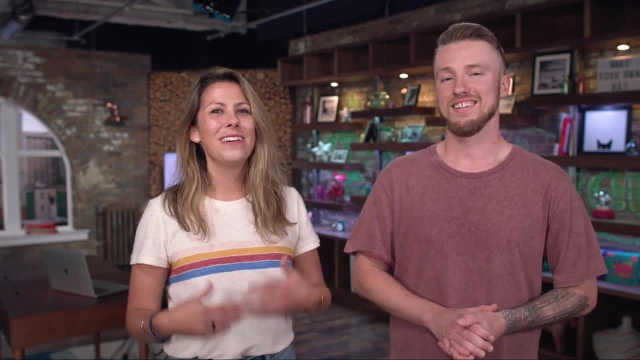 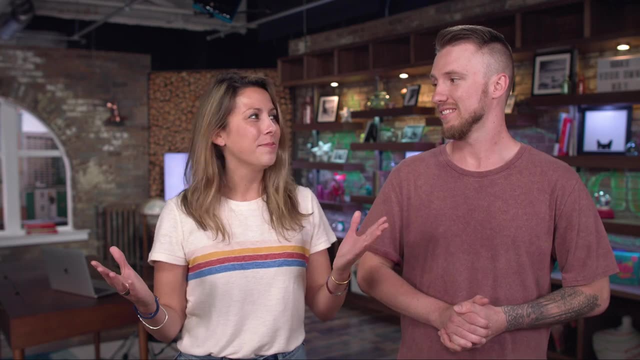 Feedback is a gift. Feedback is a gift, Yes, And so when you ask questions, you're again social, listening to help improve your brand and also what you want to do at the end of the day, your mission statement: 100%. So what's the very last tip? Number five: 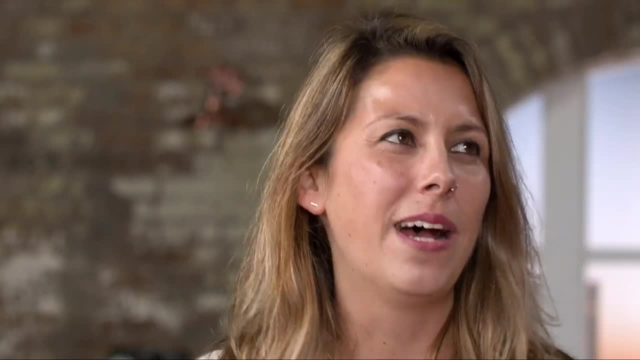 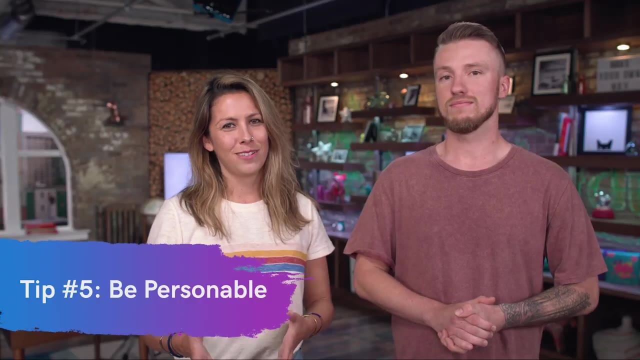 Well, okay. So number five I've kind of mentioned when I was talking about responding when Nealey and I were chatting. but number five is because we've got to place emphasis on this. This is huge. Be personable. So when I say be personable, 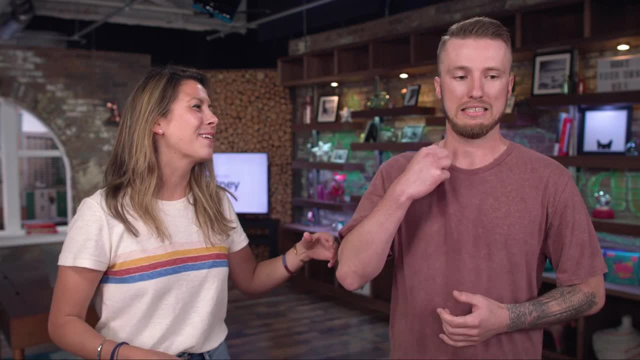 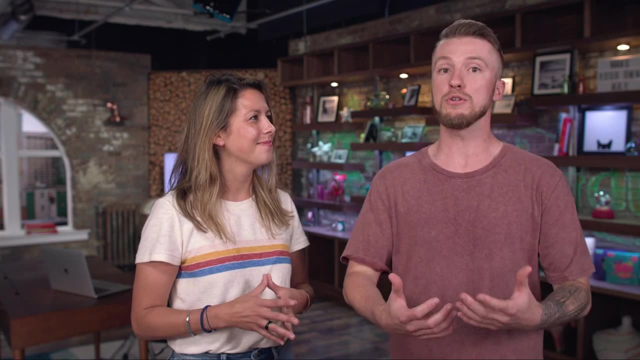 cause you're great at this, not to put you on the spot. When I say personable, what would be some best practices that come to mind to you? Just guess Honestly, it's just being you right. Everyone else has taken be you. 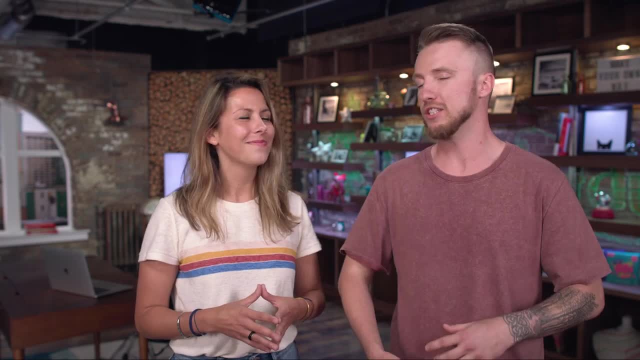 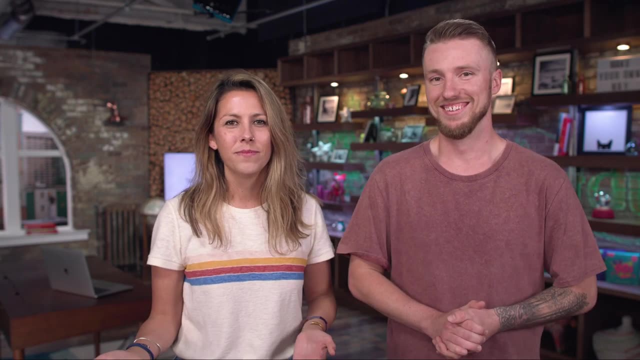 that whole cliche. Just give them a response from the heart, Not just a quick Hey, thanks, Or okay, Or see you next time. You're on the right track. Also, use their name. You know when that customer is taking the time to respond to you. 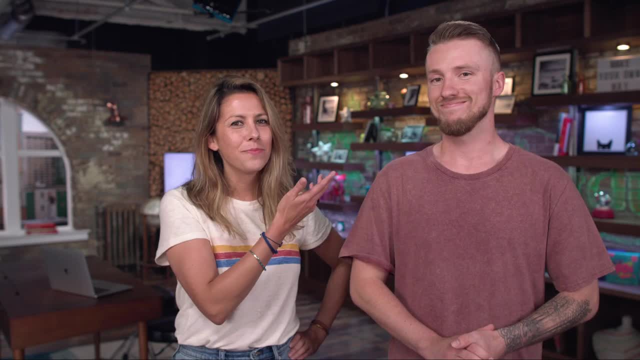 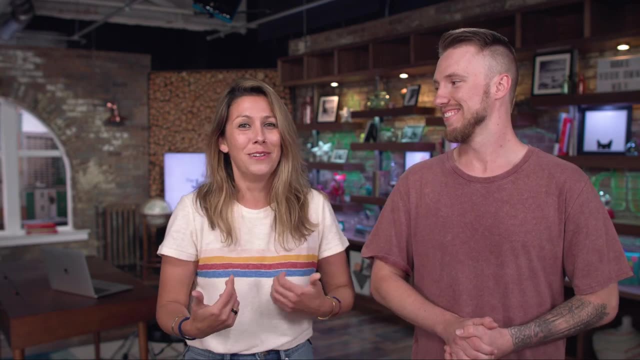 respond back and use their name. I mess up his all the time because he goes by Justin, but he also goes by Nealey. I know all you viewers out there I've been called worse. You go by Nealey, but either way I use one of those names, So I'm being personable. 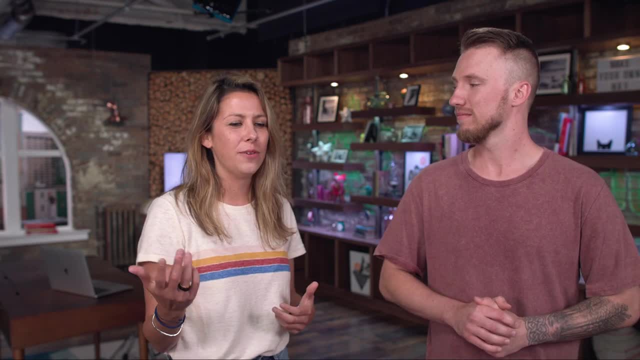 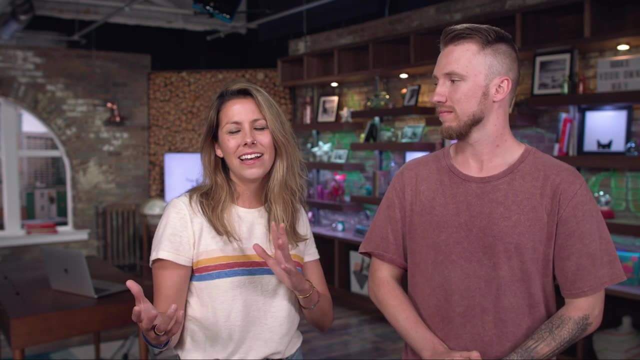 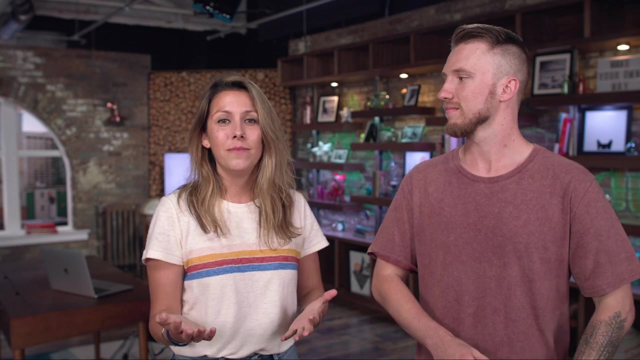 I'll also include any details that they included. So if they went into your carwash and they talked about how efficient it was at getting a spot, free rent and all the amenities that you have, or they go to your salon and everyone was so personable and he got a complimentary glass of champagne and they loved that, 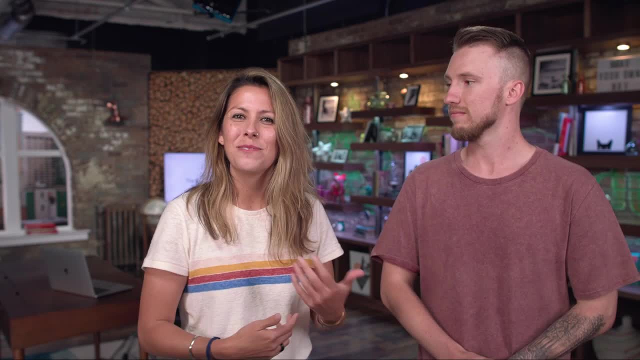 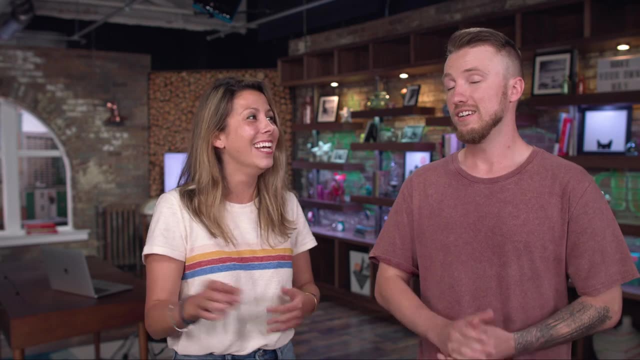 about it. We'll include that detail when you respond back and that shows that you're actively listening, which really ties it all in all five. It's like a circle and just a bonus for you Like sometimes someone may not mention you directly. 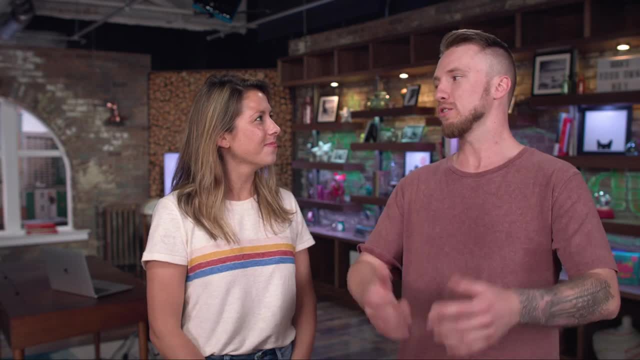 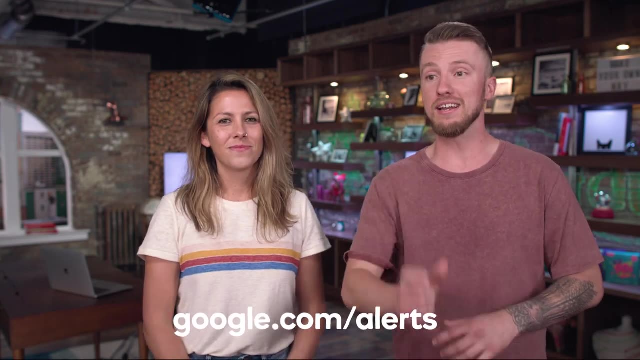 They may not tag your business, They might just be venting on social media or talking about you on social media. There's a site called Google Alerts. you can literally go in and put your company name in, and every time it's mentioned on a website you're notified.